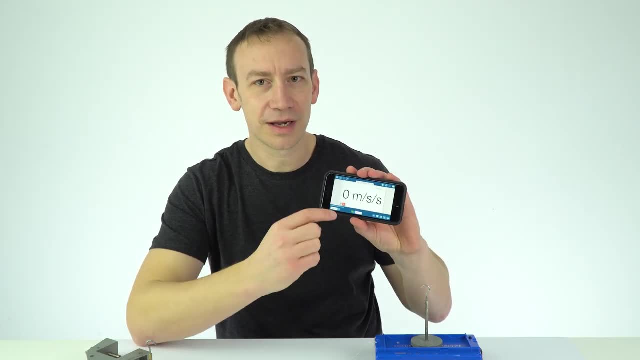 to my phone and then what this is going to do is directly give me the maximum acceleration of this cart as it's running. So I'm going to go ahead and do that, and I'm going to go ahead and do the same thing with the other cart and the same thing with my cart. so we're going to go ahead and 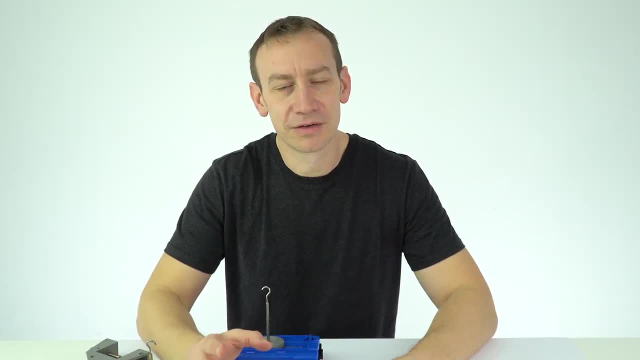 do this just like this, because we're going to do this on the table and it's moving along the desk, So we can read off the value for the acceleration, we can calculate the size of the force and then we can look at how these two variables are dependent on one another. Now it's really important with 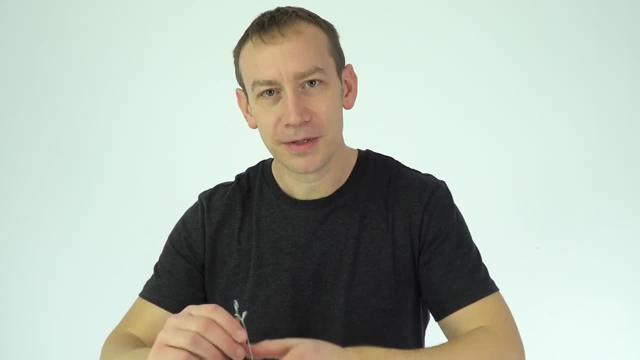 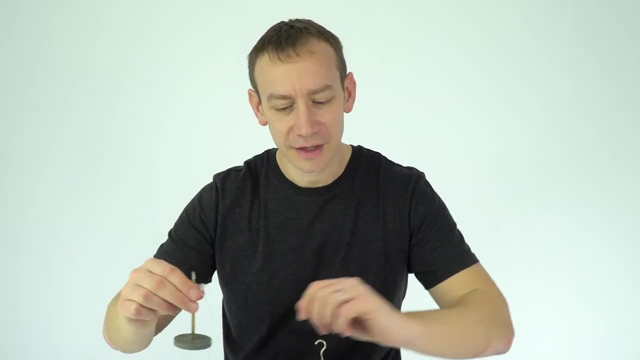 this experiment that we keep the mass constant, and we're going to be doing that by attaching other masses on top of the trolley, because what's accelerating isn't just the falling mass, it's also the trolley which is going to be accelerating across the table, and this is the thing that's being 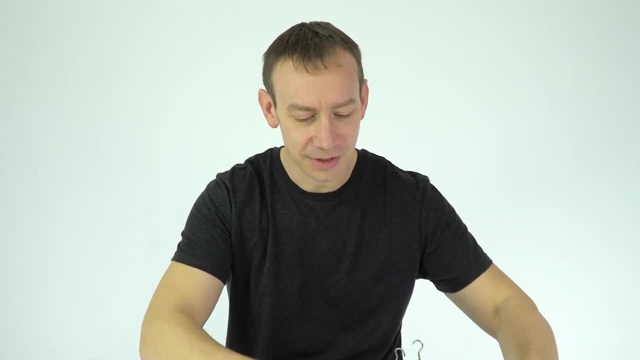 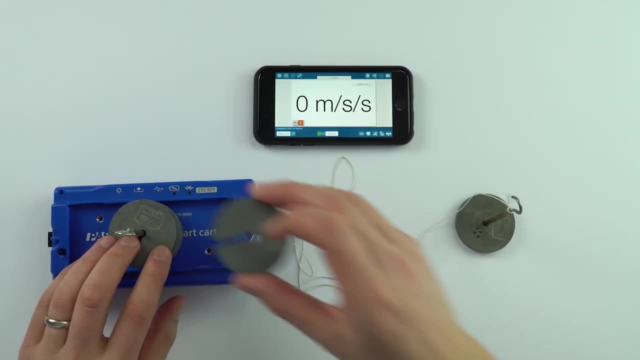 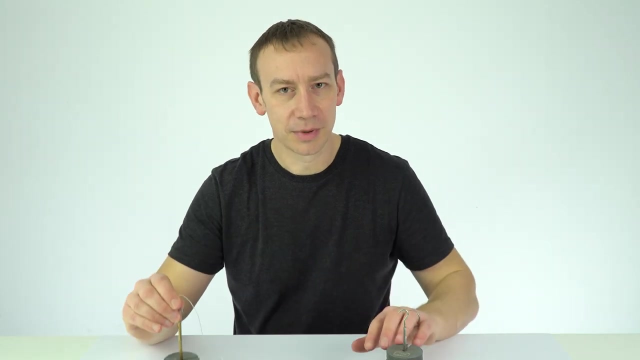 accelerated this total mass. Now that's really important, and we can keep that constant by keeping these masses here on the trolley when they're not being used, and then we transfer them onto the falling mass. Now what that means is we are changing the force that's being applied to this trolley, but the 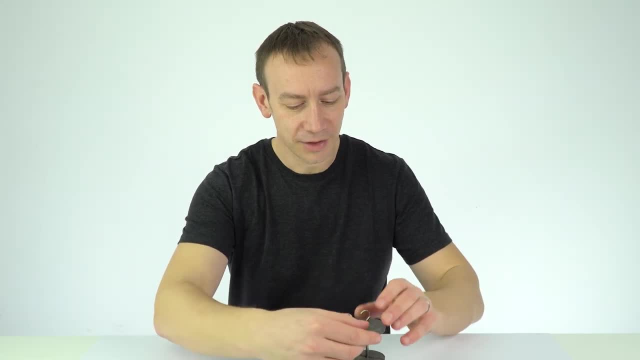 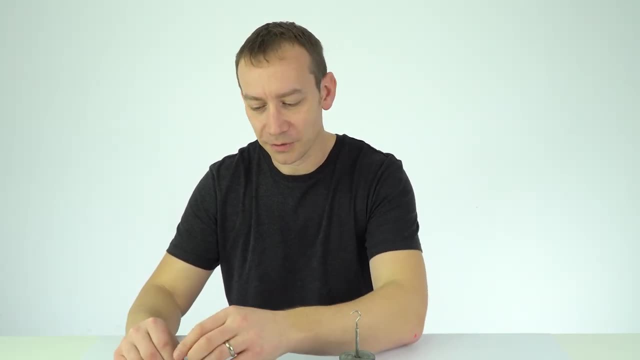 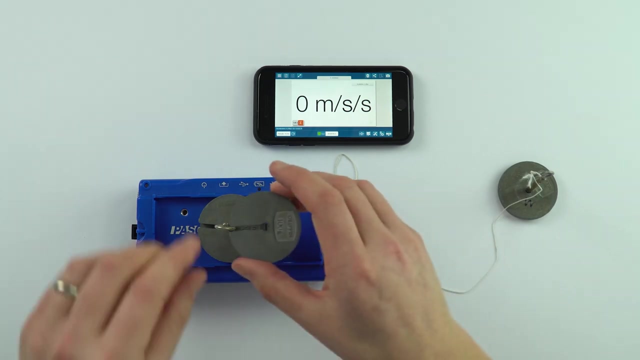 total mass stays the same, because all we're really doing is taking a mass from here and we're just putting it onto there, So the total mass stays the same with changing the force, and that's really important. Now, the first value we're going to take is when we have a force of zero newtons. 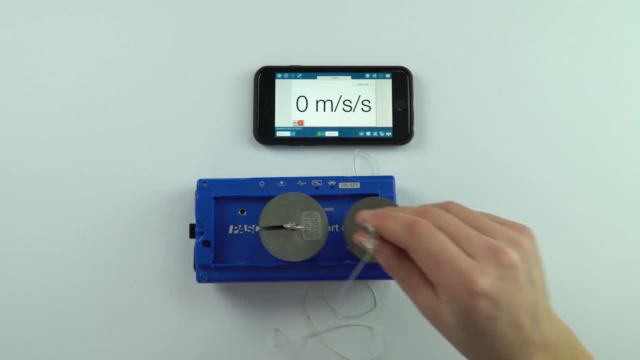 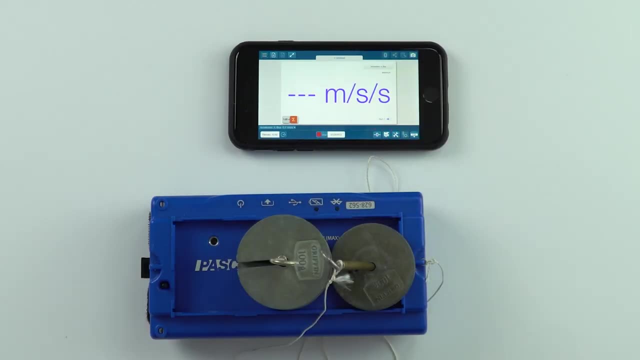 Okay, so I'm just going to put this mass on top of the trolley, like so, and with the data logger, this is going to give us the reading for the maximum acceleration. So I'm going to press start and I suppose that should really be zero, shouldn't it? So let me just zero that number. 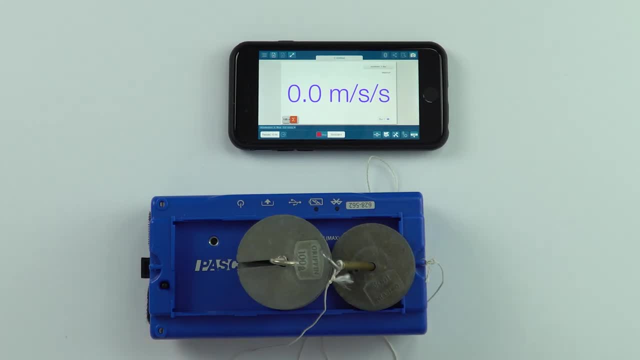 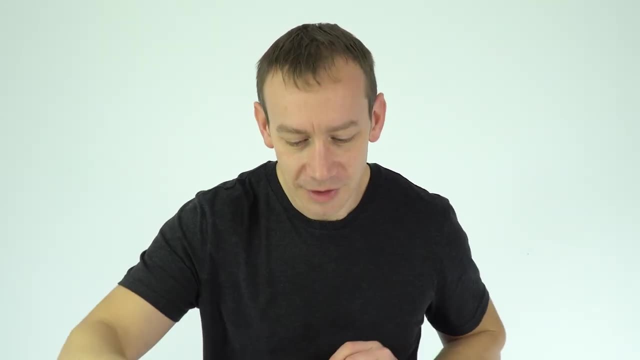 So yeah, the first reading when we've got no resultant force is zero meters per second squared. That's kind of what we'd expect. There's no resultant force, there's no acceleration, So I'm going to stop that reading. So we've now zeroed it as well. 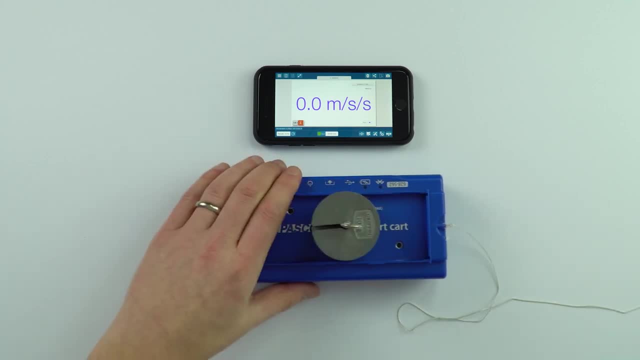 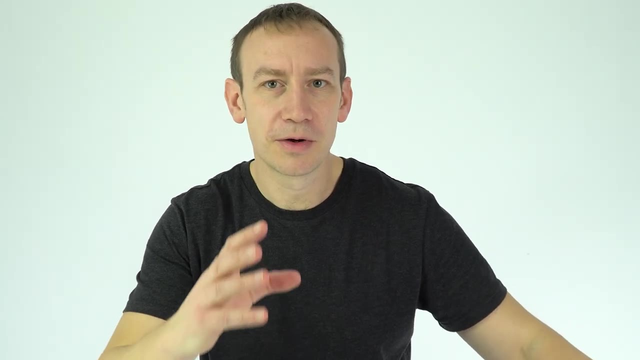 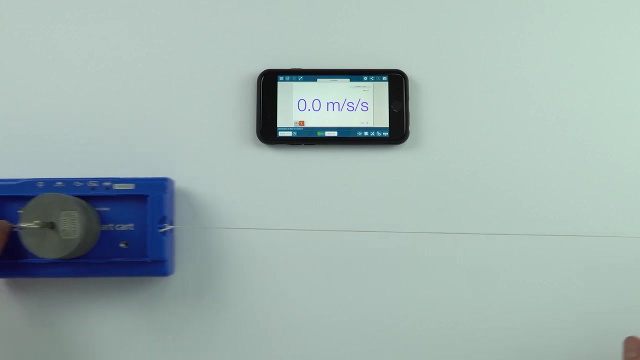 I'm now going to hang this 100 grams over the end of the bench, Okay, and the important thing here is that we're only going to be recording the acceleration, as that mass is falling. At the moment, this is the highest point where it's near the table, and if I just push this or let it go, 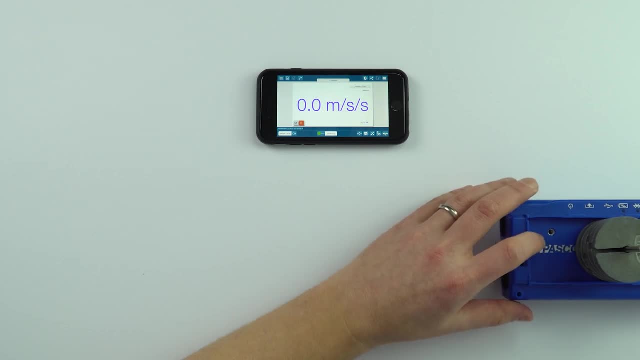 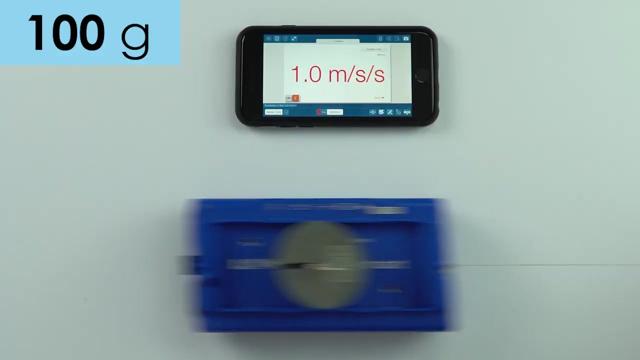 to about here. this is the point where the mass is now on the floor. So, basically, this is the length of the experiment that we're going to be using, So I'm going to pull this back very slowly until the mass is at the top. I'm going to press start. So that's our first reading With 100 grams, which 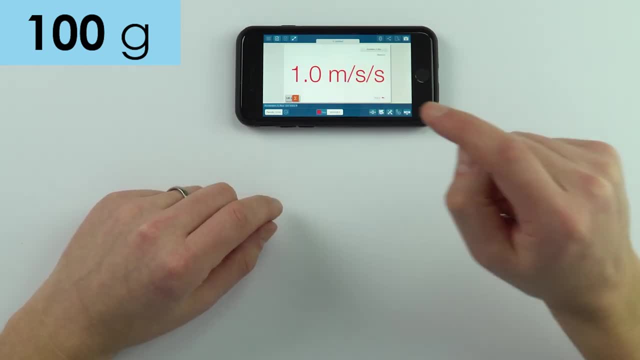 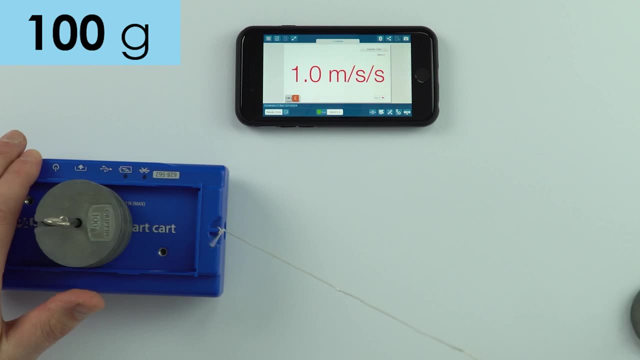 is about one newton. we've got a value for the acceleration of one meter per second squared. So I'm now going to go to the next reading. So I'm going to go to the next reading, So I'm going to take this mass, I'm going to take one of these, I'm going to put it on there. So we now have 200. 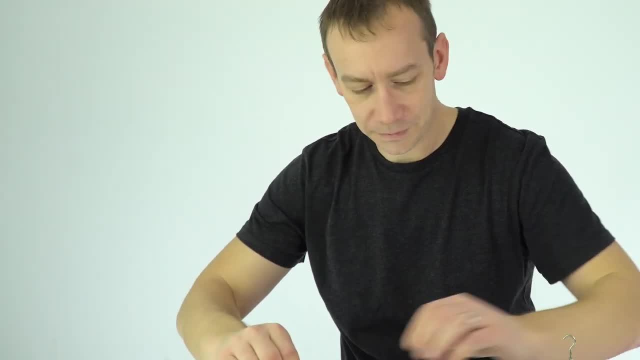 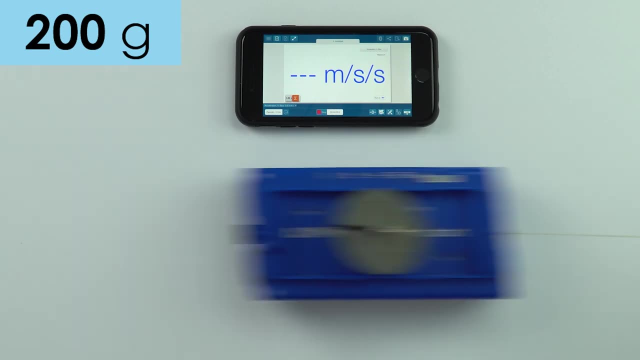 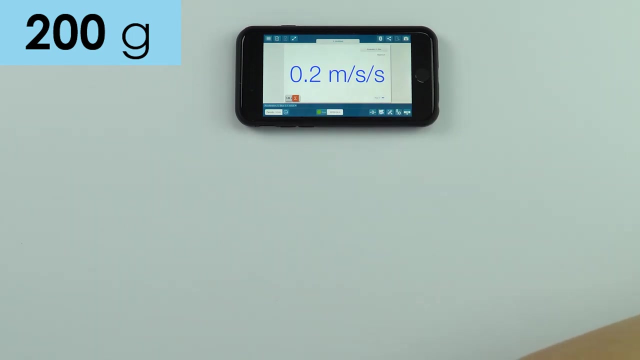 grams overhanging the edge of the bench. I'm going to put this back to here. I'm going to line it up, I'm going to press start And we've got 0.2, which might be an anomaly, So I might do that one again. 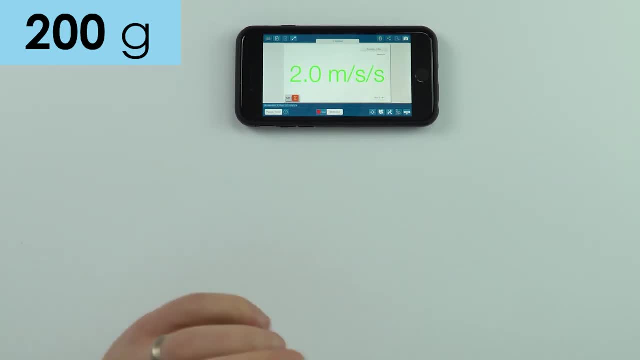 Okay, that looks more like it: 2.0 meters per second squared. I'm going to do the same for 300.. That one gave a value of 3.0 meters per second squared. Data is looking pretty good so far, So we're now going to do it for 400,, 500 and 600. 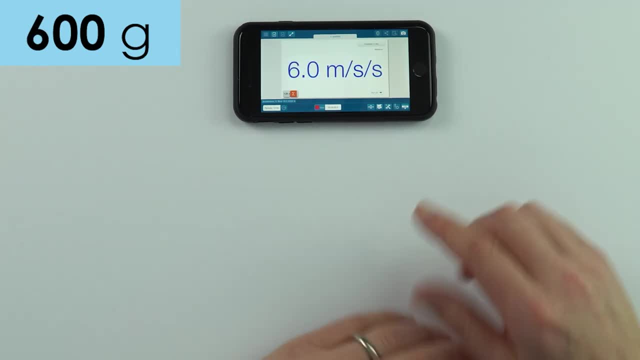 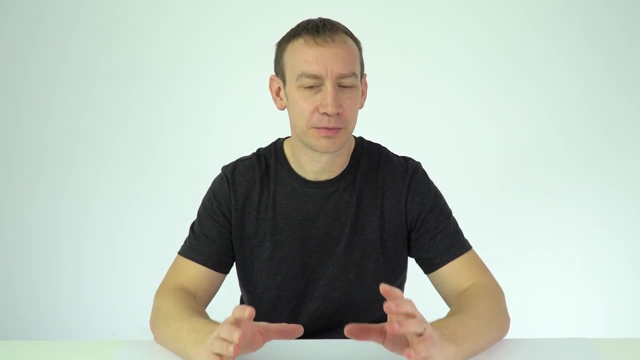 And how about that? A pretty good set of data actually. So with that last one, we had 600 grams and we got 6 meters per second squared. I think there's a pretty strong correlation between these two sets of data. So what we can now do is we can plot this on the graph and look at the relationship. 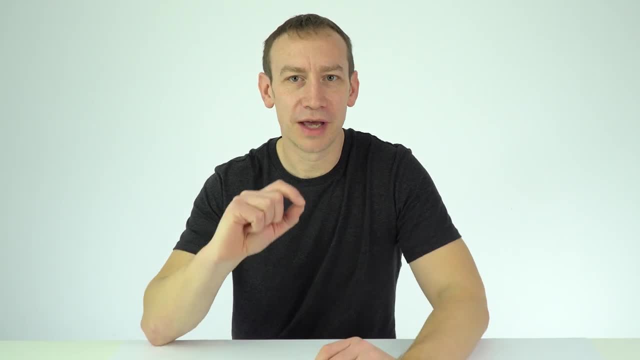 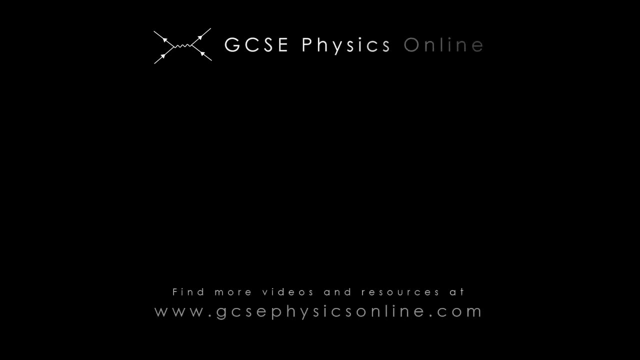 between the acceleration and the force applied when we have a constant mass. So that data, we're now going to plot the mass in terms of the relative mass to be a constant mass. So that's what we are, and now we're going to plot it in terms of the relative mass. I'm going to do it at 0.5.. I'm going to put my scale down at 0.5. And I'm going to do- I'm going to put mine below this rated value. And now I'm going to plot that over here. I'm going to plot that over here. Okay, That's good. OK, That's good.